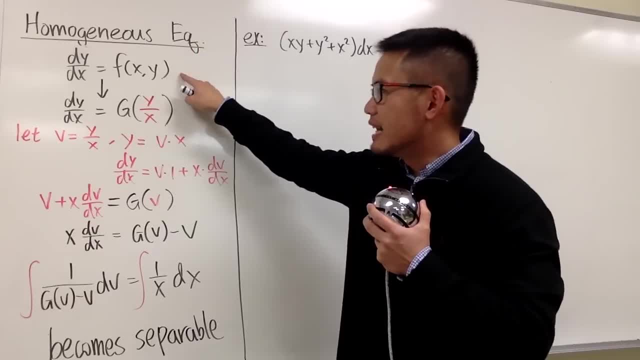 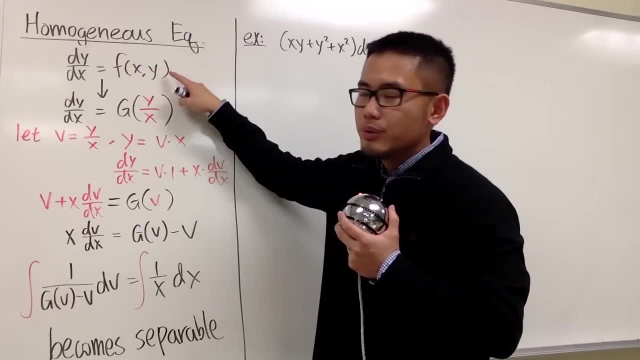 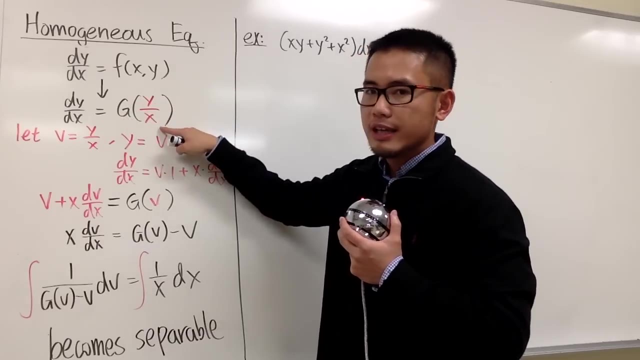 And suppose this is not linear, this is not exact, this is not separable. Then try the following: Try your really best to write this into an expression that's in terms of y over x, And we will now call this to be g of y over x. 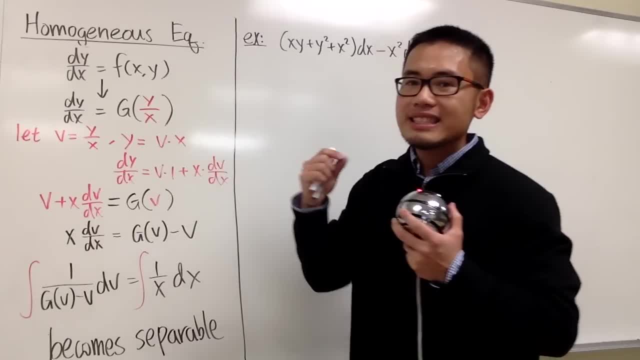 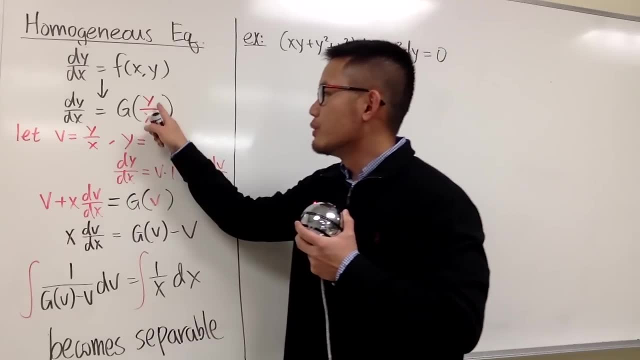 And once again, y over x has to be together and that's the one input. okay, And if we can make this happen, next what we are going to do is we are going to let phi just another variable, and usually we call this to be phi. 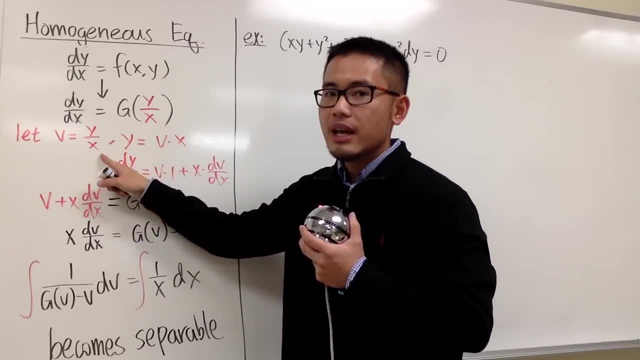 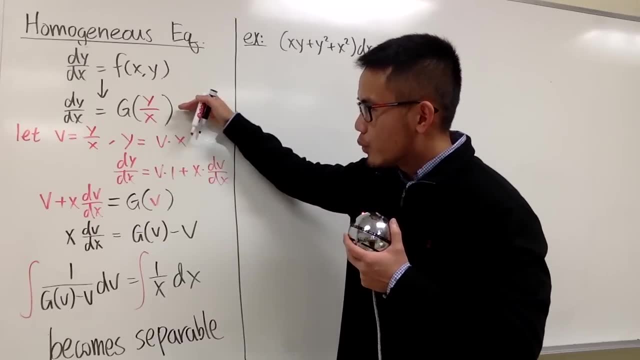 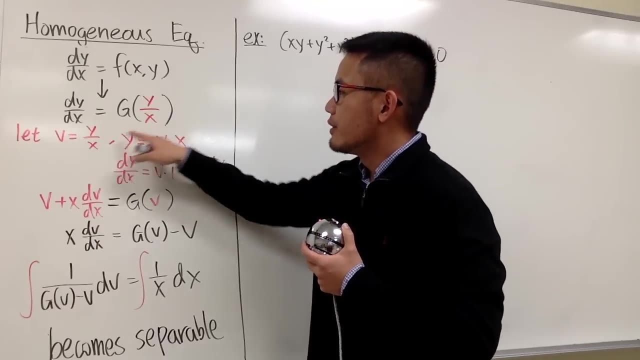 We let phi equal to y over x, and then we have to figure out what's dy dx in terms of phi as well. So that way we can take this differential equation into a differential equation that involves phi and x only. So right here, phi is equal to y over x. 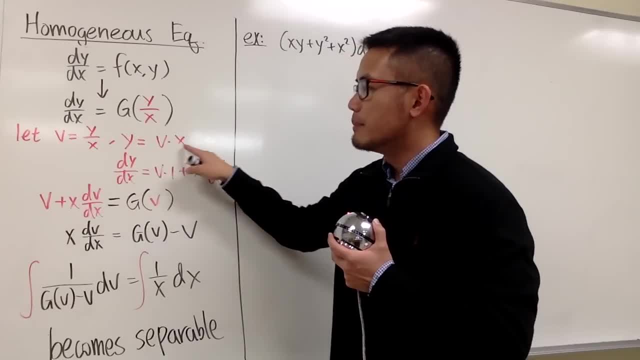 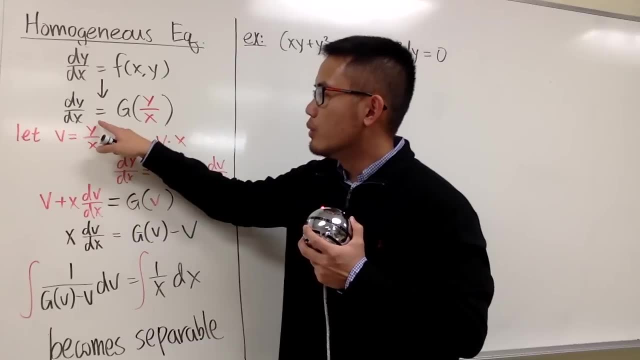 Let's multiply x on both sides, So we have: y is equal to phi times x, And notice that y is a function of x. x is of course a function of x. phi is equal to y over x, So of course phi is also a function of x. 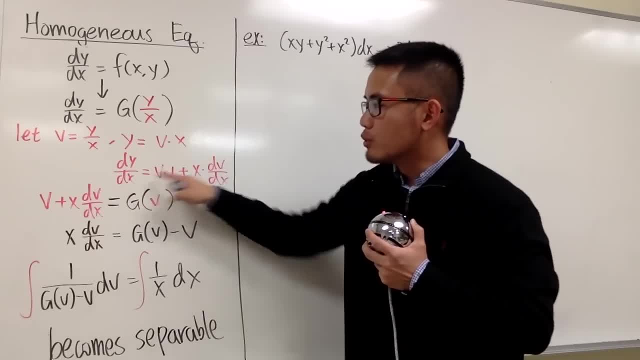 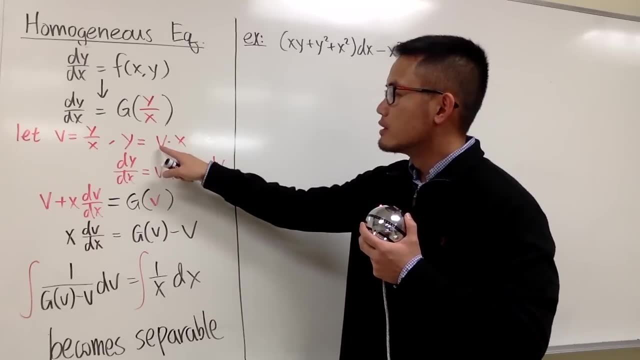 Since y is equal to phi times x, we differentiate both sides. The left-hand side is dy, dx, that's it. But then I'm going to write this: On the right-hand side, we have to use the product rule. So we keep phi and the derivative of x is 1,. 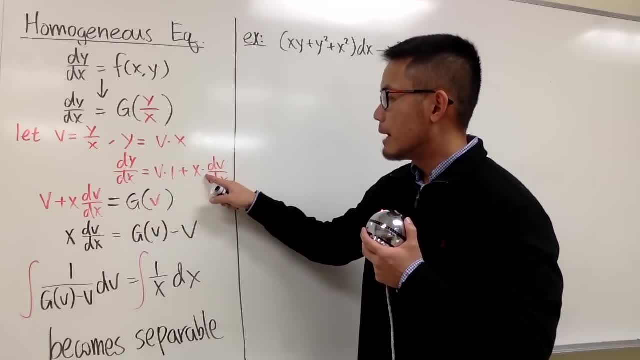 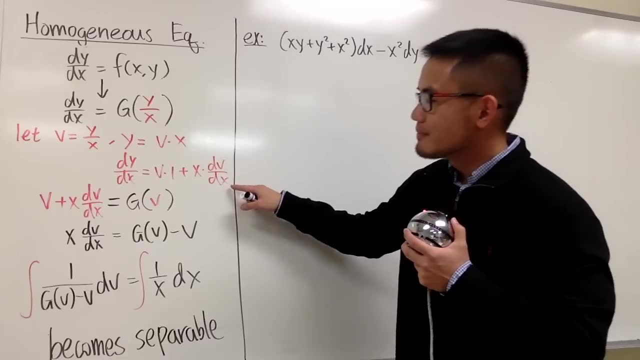 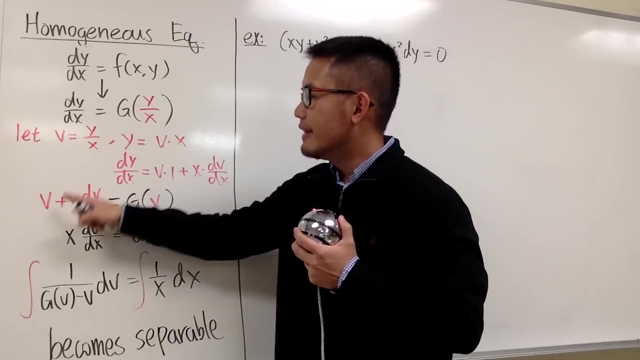 and then we add it with: we keep x and we multiply by the derivative of phi, which is dv dx, because phi is a function of x. So this, right here, is what we are going to use to replace dy dx, and now we have phi plus x, dv dx. 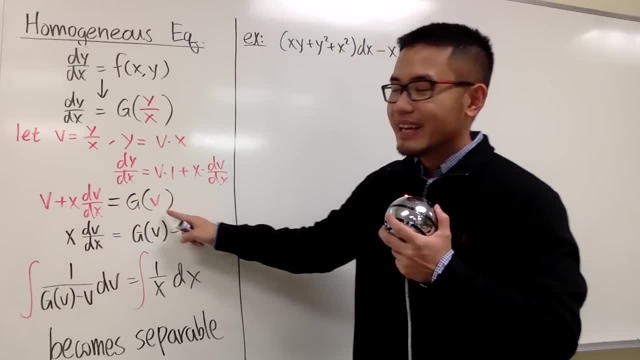 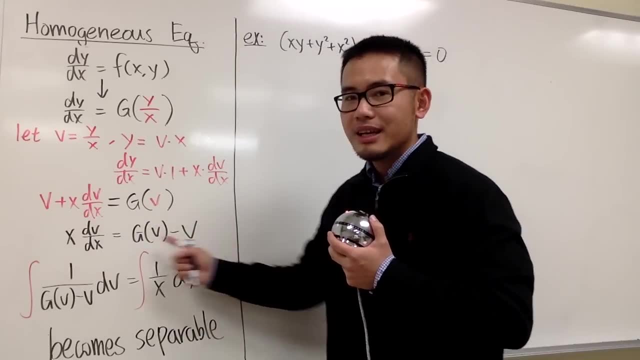 and this will be g of phi. And now, once we have this right here, we can subtract v on both sides and we have g of phi minus v on the right-hand side and x times dv dx on the left-hand side, right. 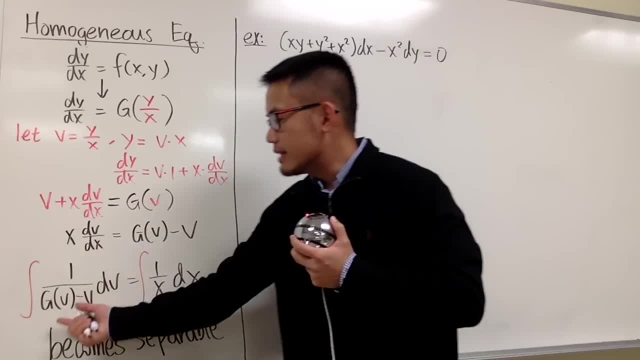 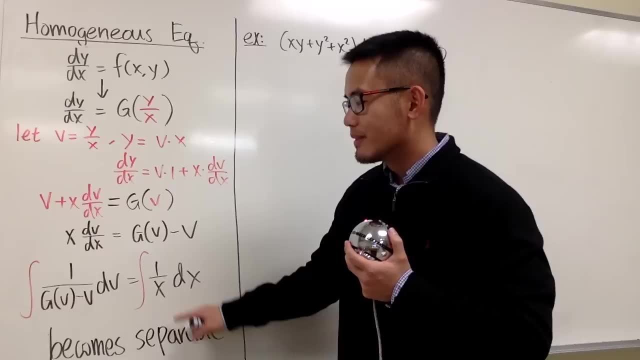 We can divide g of phi minus v on both sides, and that's what we have, And that's multiply dx on both sides. and then we have to divide by x on both sides, so we have 1 over x. And you see, now this becomes separable, right. 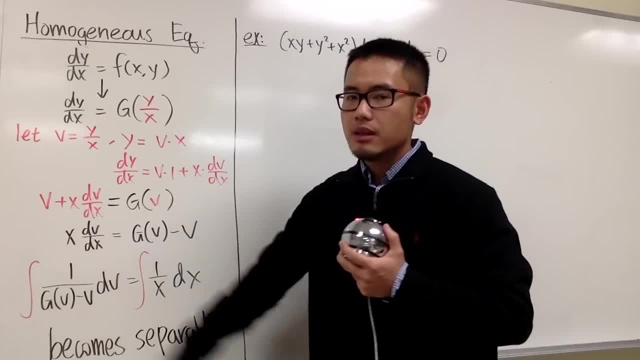 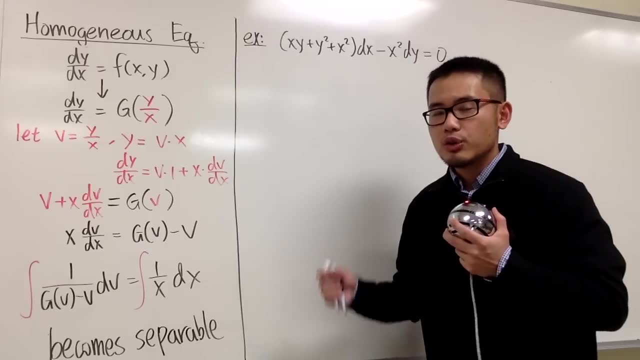 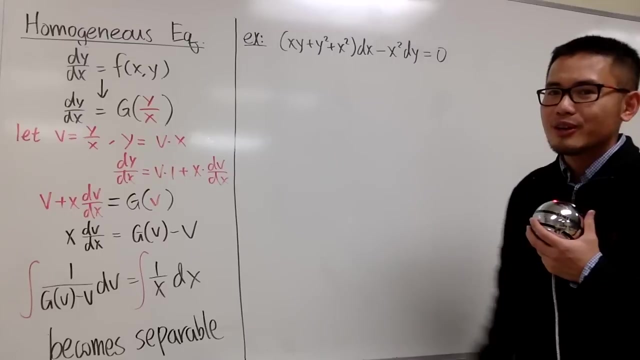 It becomes separable. if you have that- And of course this is separable- we can solve it. and after you solve that, just make sure you write your answer in terms of y and x at the end. Let me use this to demonstrate the steps right here. 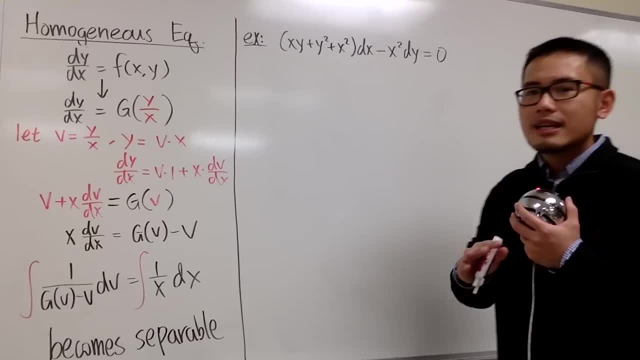 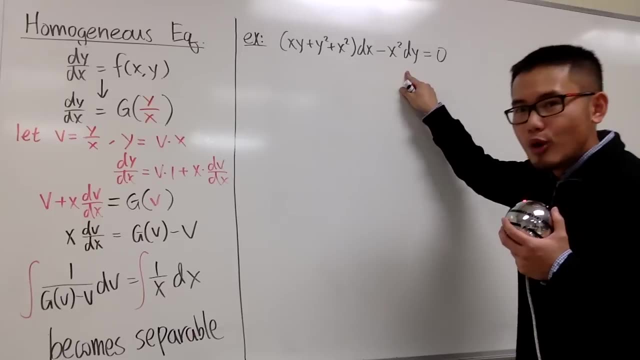 So this is what we have, and let me tell you, this is not separable. this is not exact, this is not linear. okay, This is not separable at the moment, but I will make it into separable because I can do that. 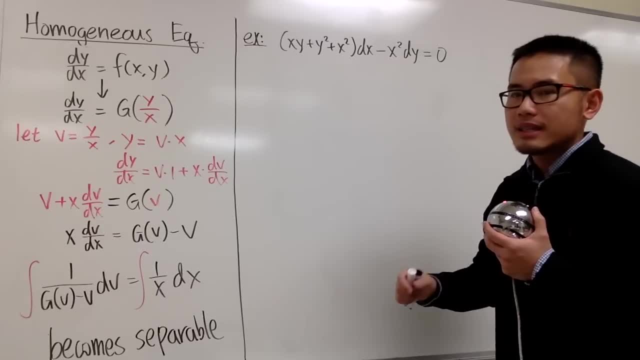 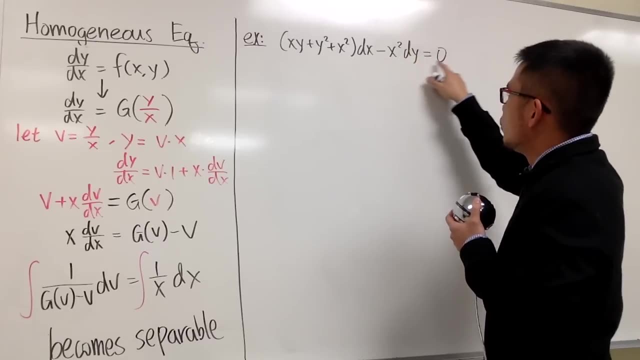 Okay, so I'm going to rewrite this in terms of dy, dx, equal to whatever, right, So I want this form. Let me add x squared dy on both sides, but let me put it down here first, though, So we will have x squared dy, positive, okay. 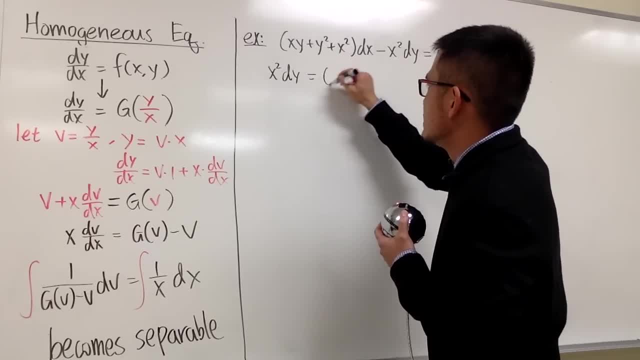 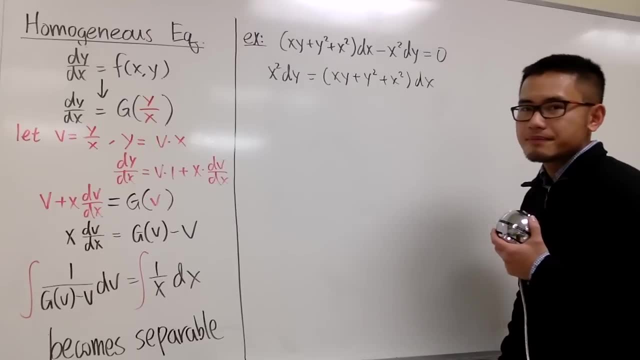 And then I'll keep this on the left-hand side, but I will make this still positive: xy plus y squared plus x squared dx. okay, Okay. So once again, I just move this to the right-hand side so it becomes positive. but I put that down first. 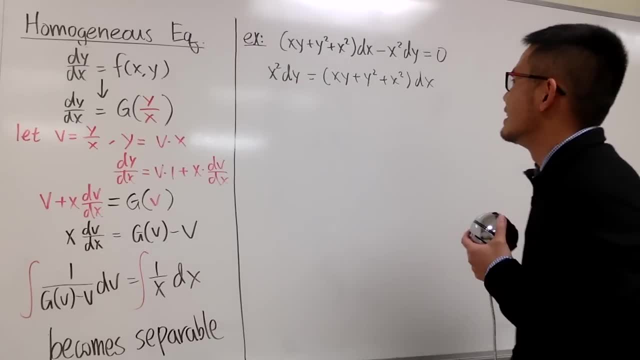 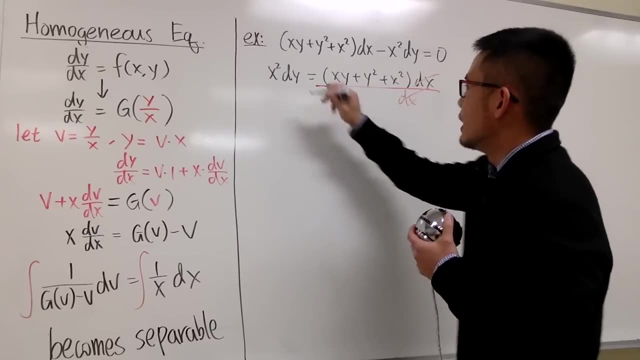 because I want to have the dy on the left-hand side. Next, I'm just going to divide both sides by dx right- The usual business. so they cancel. I'll divide by dx right here as well, so I can get a dy dx. 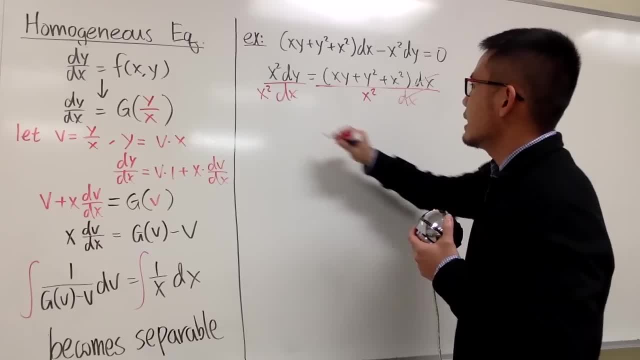 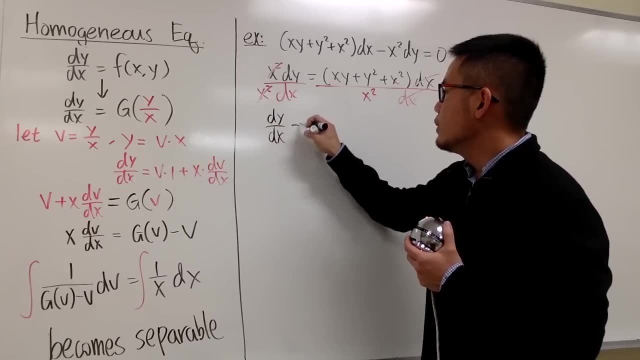 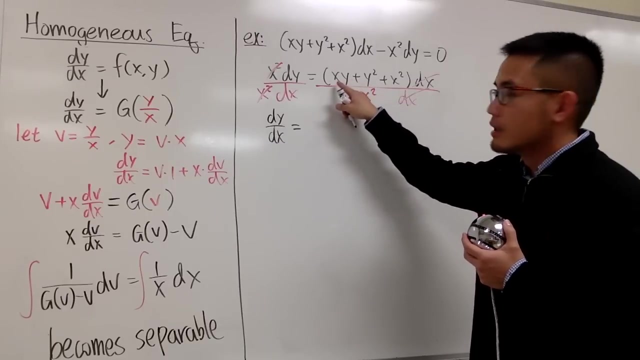 but then I will have to divide it by x squared, like that, so that this will cancel And we will see this is dy. dx equals to: and now let's simplify this carefully: We have xy over x squared, so we will get the x cancelled out. 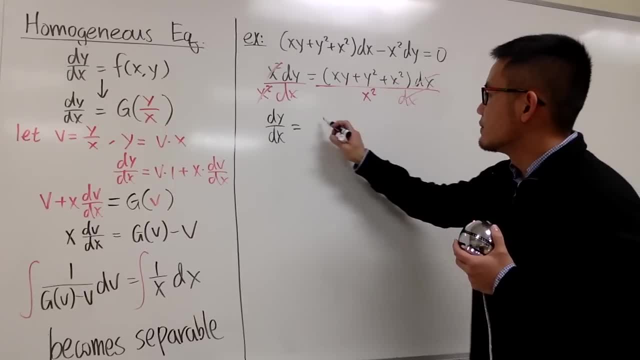 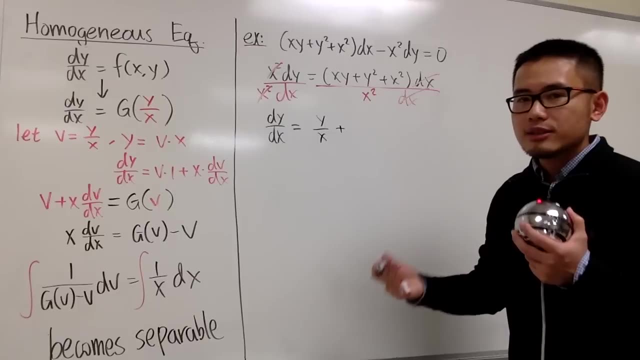 but we still have one more x on the bottom. We will have y over x first, and then plus. this is y squared over x squared, and that can be cancelled out, right? However, let me look at this as y over x. 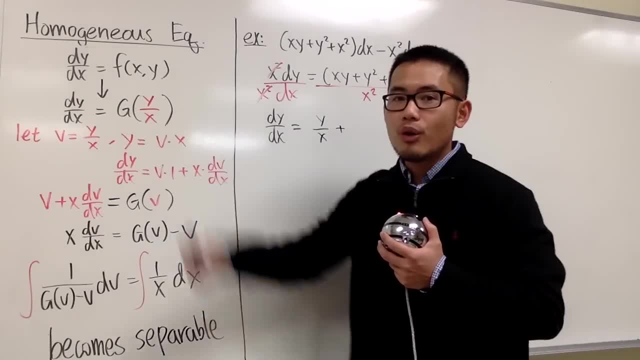 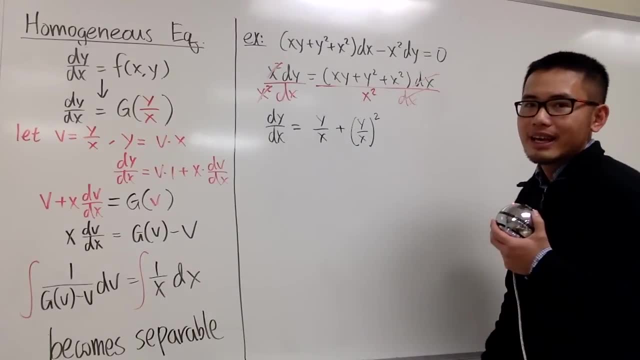 and then squared, because I want to have in this form: okay, So let me rewrite this as y over x and then squared At the end. x squared over x squared is just 1, so plus 1,, like this: 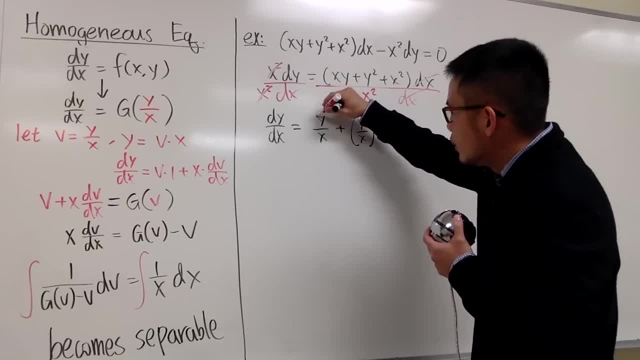 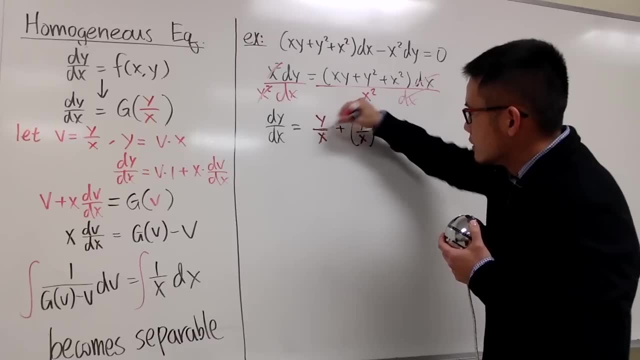 And you see, on the right-hand side here we have y over x and then this right here is also y over x, right? So, as you can see, y over x are together and that's pretty much the input, So we can do this right. 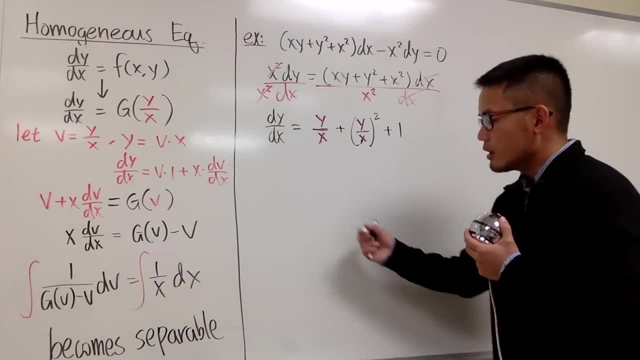 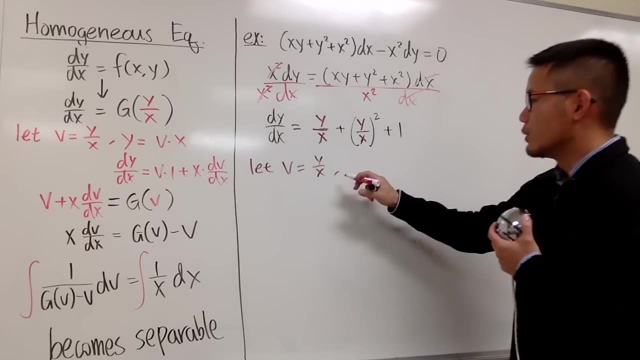 Because we achieved it. we're going to do the following. So here we go. we are going to say: let v equals to y over x, and of course it's pretty much all that. so we can just. well, let me just do it again. 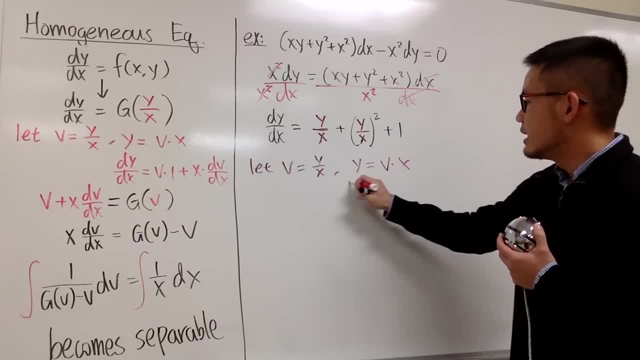 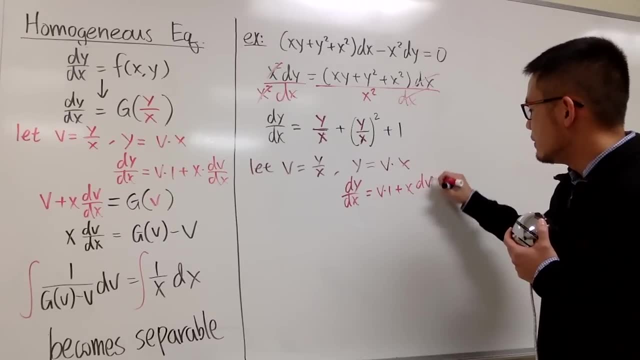 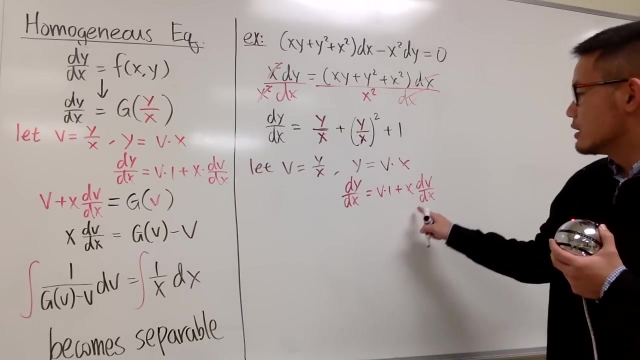 y is equal to v times x. and then you know, dy dx is equal to v times 1 plus x, dv, dx. Suppose I didn't have that on the board, I have to do this again, right? But anyways, replace this with dy dx. 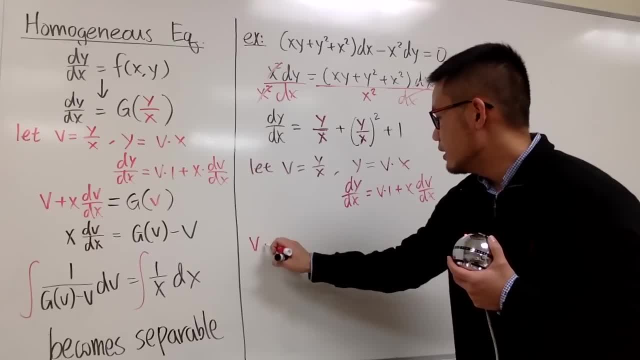 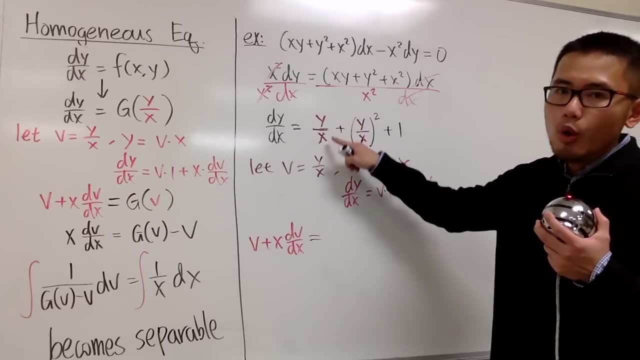 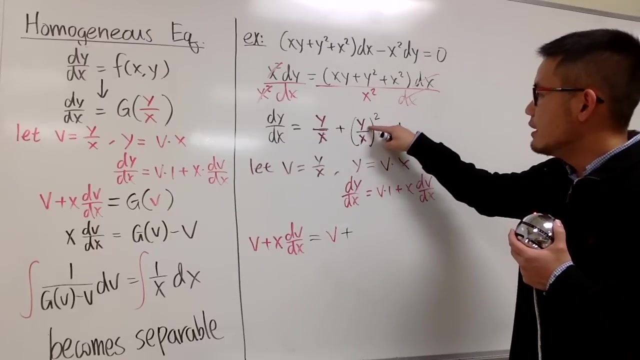 and now that's what we get. On the left-hand side we have v plus x, dv, dx, and that will be equal to y over x is v, so we have that equal to v, And then we add it with: this is v, and then squared. 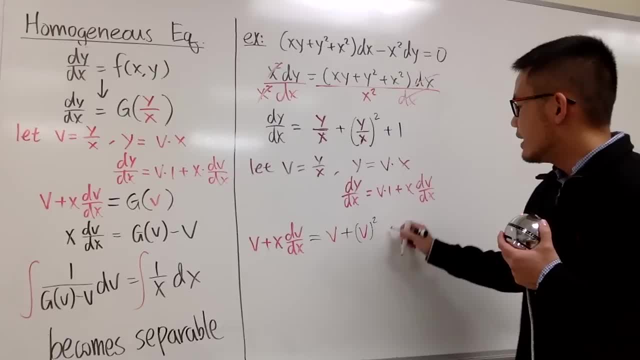 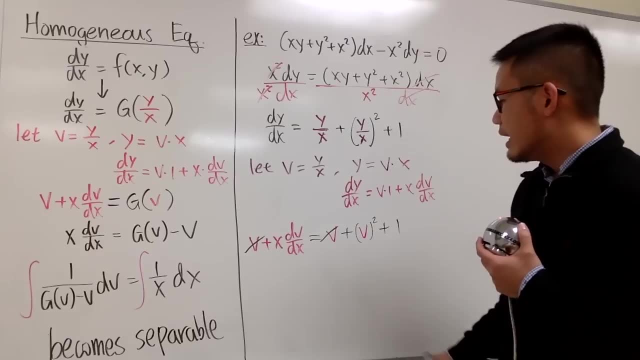 so we have v squared like this, And then we have the plus 1 after that. Okay, you see we have v here, v here, so these two v's cancel, and let me just divide this on both sides. 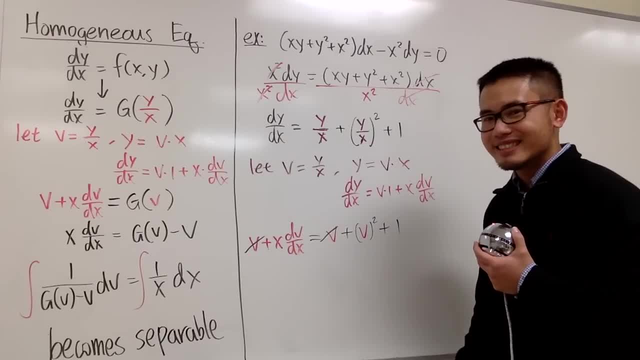 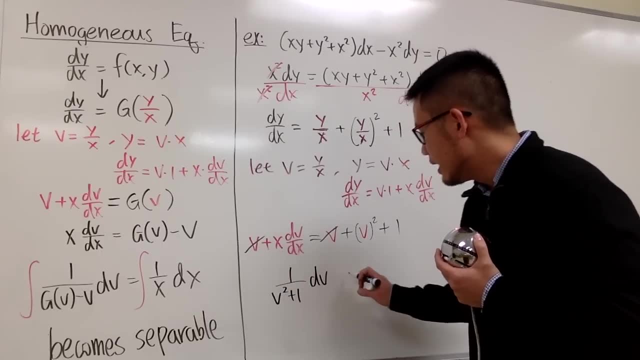 and then let me just divide the x on both sides. multiply the dx on both sides. On the left-hand side, we'll end up with 1 over v, squared plus 1, along with the dv, and this will be. we divide the x on both sides. 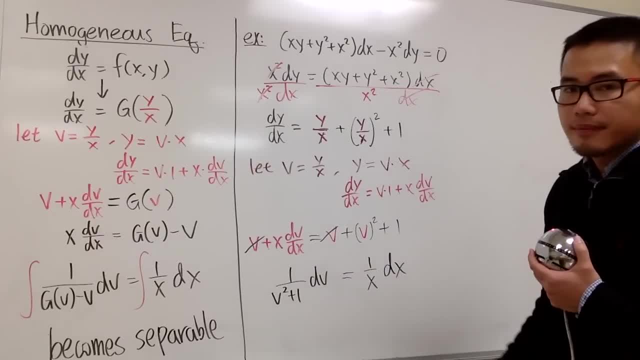 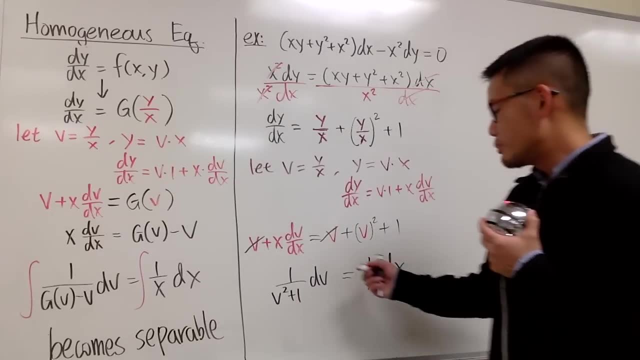 so right here, and then we multiply the dx on both sides, like this: And then of course you see all the v's and dv's are together and all the x and the dx are together. Just separate it, Integrate, integrate. 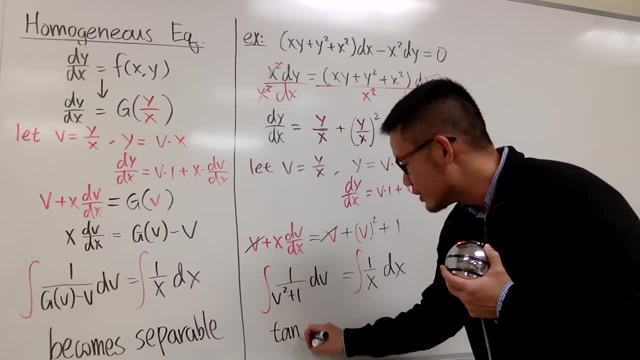 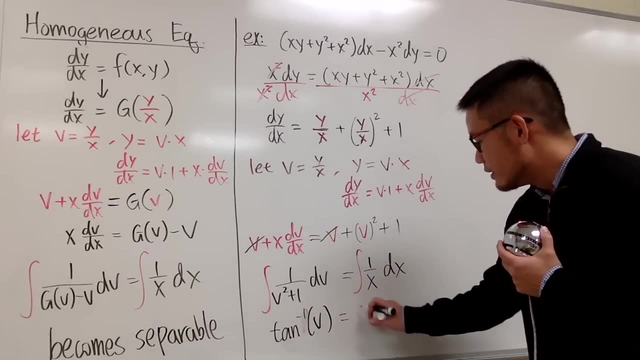 On the left-hand side we have the inverse tangent of v, Right This right here is the inverse tangent of v, And on the right-hand side we have the natural log absolute value of x, And then we put down plus a constant.